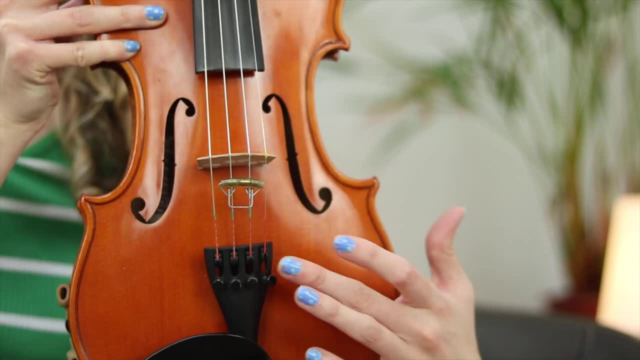 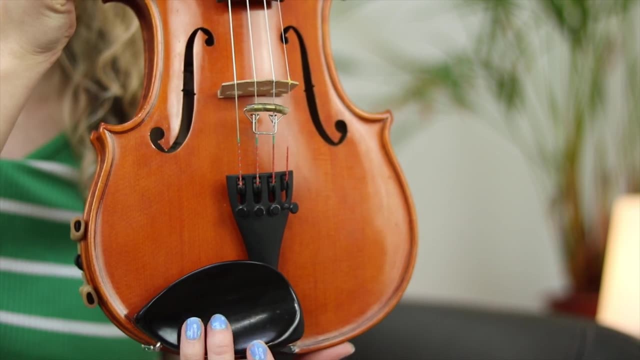 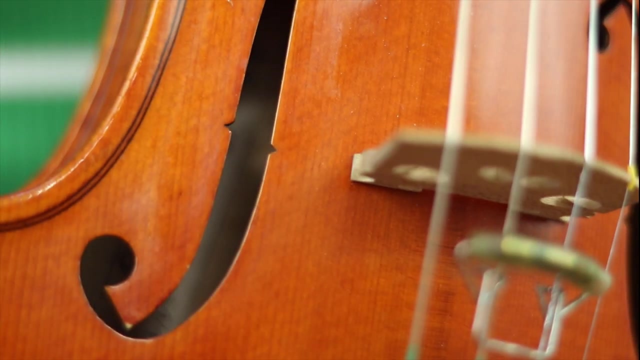 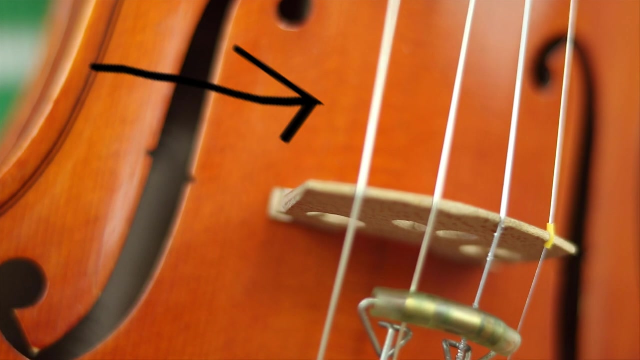 bridge, the tailpiece and the chin rest. Can you guess what part of your body, the chin rest goes underneath? Finally, we have the F holes. Let's take a closer look. These F holes is where the sound of the violin comes from, When the string. 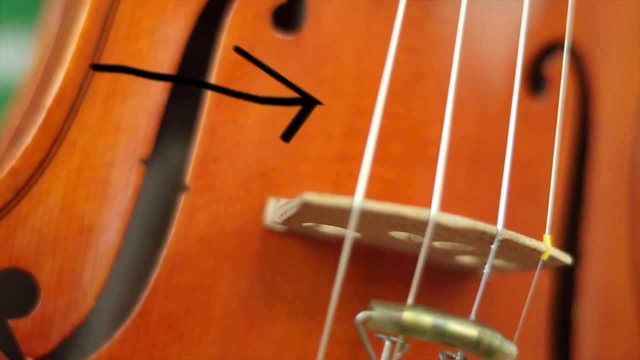 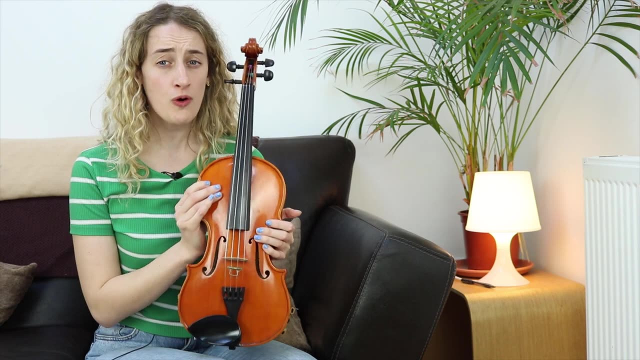 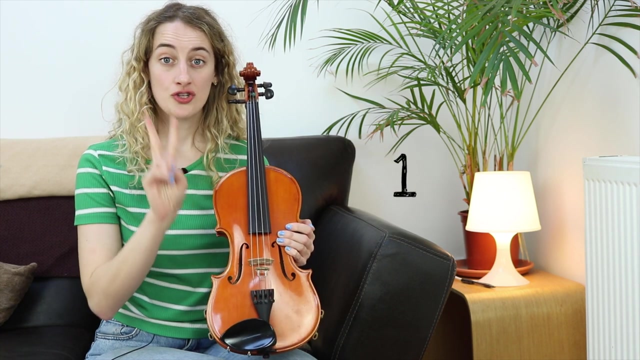 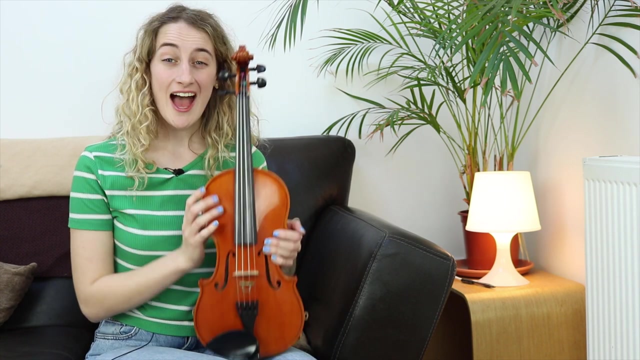 wobbles. the sound travels through the F holes and into your ear. Finally, we have the strings. There are four strings on my violin Shall we count them together: One, two, three, four, Four strings, and they all have different names. This is G. 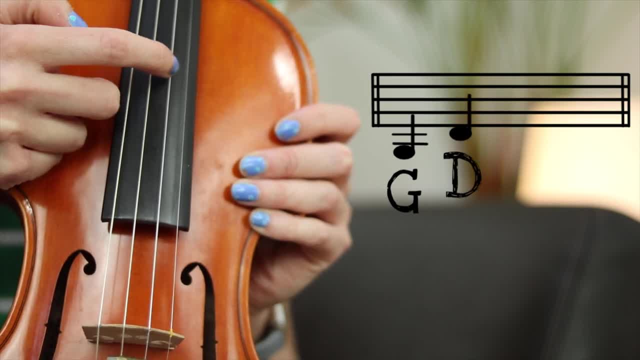 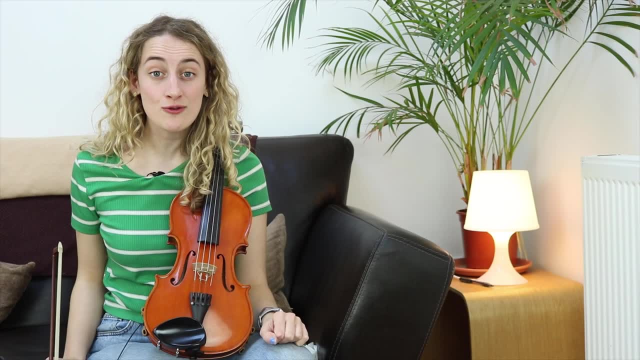 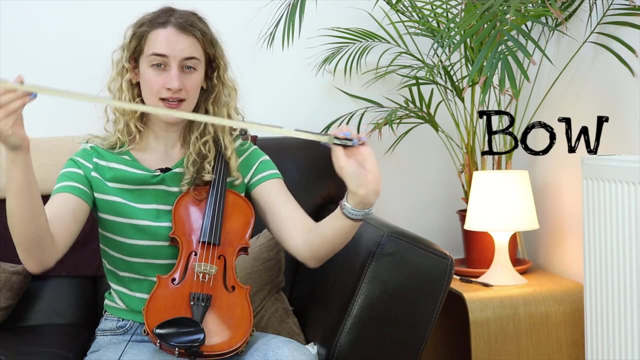 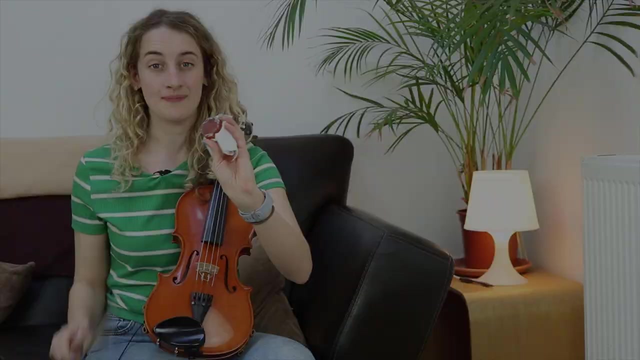 this is D, this is A and this is E. To play my violin, I need to use my bow. This is my bow. It's made of wood and horse's hair. What sound do horses make? To make a good sound with my bow, I need to use rosin String. players put rosin on their 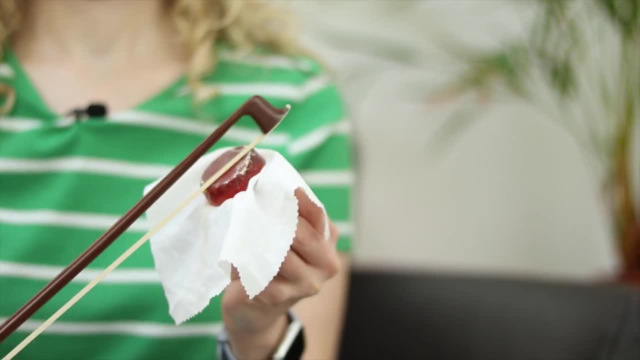 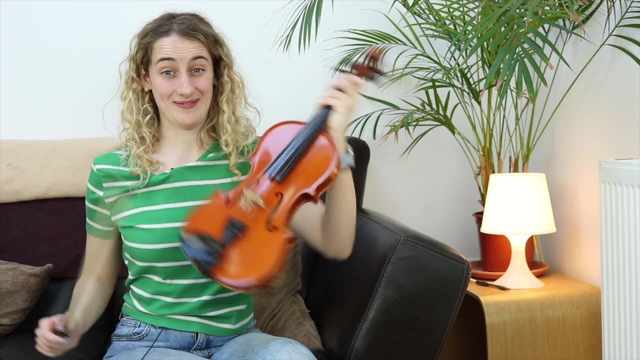 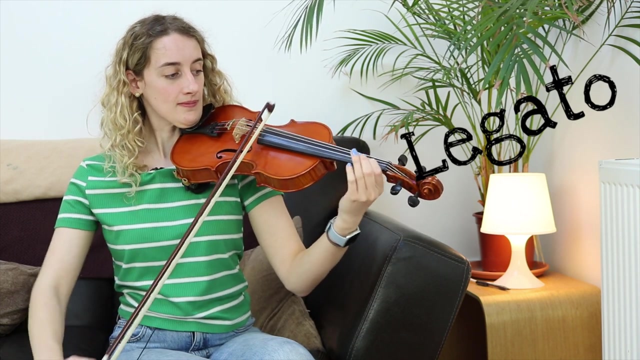 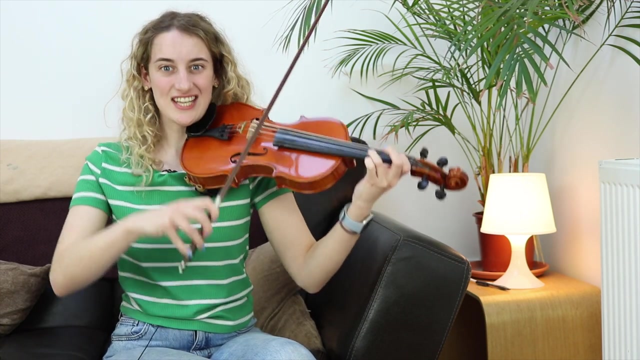 bows to make them sticky. The horse hair needs to stick to the strings to make a sound. Now let's have a listen to all the different ways I can play the violin. I can play smooth and legato. I can play bouncy and staccato. 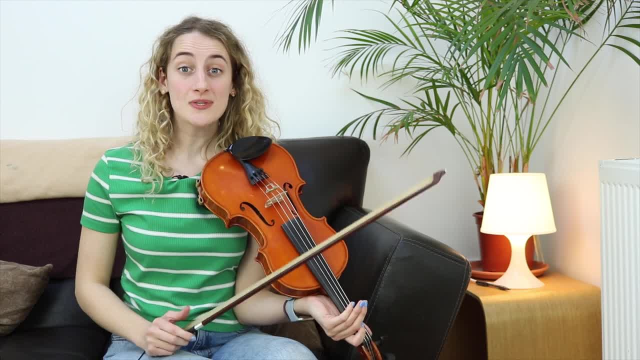 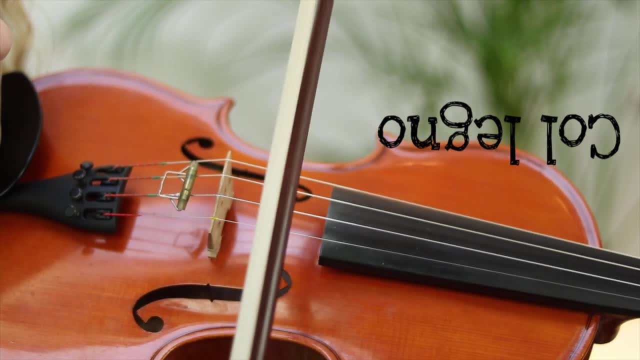 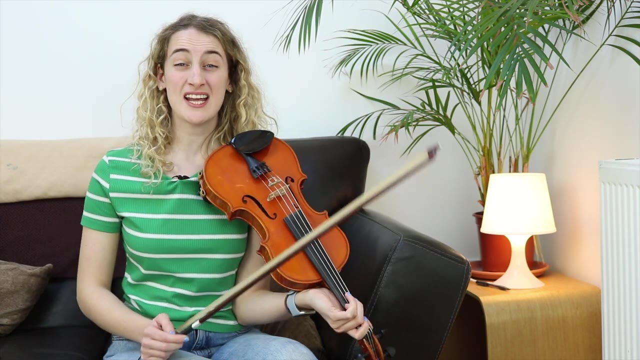 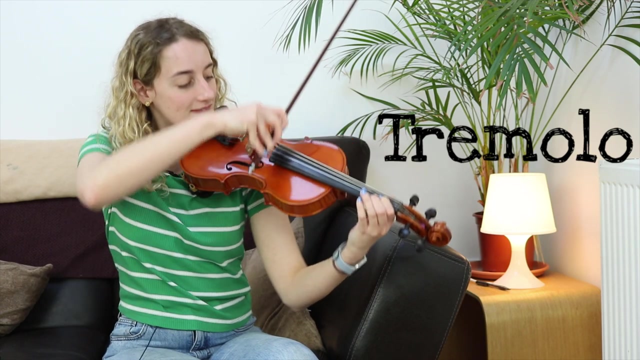 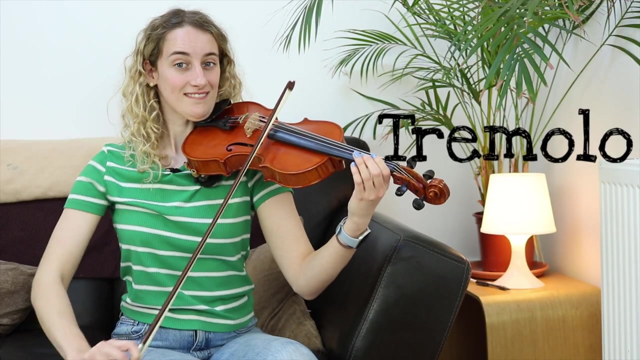 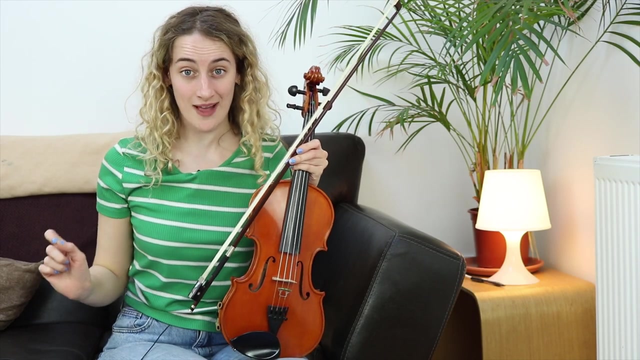 I can turn my bow upside down and play Col Legno, And I can play tremolo, which is really really fast, And I can play tremolo, which is really really fast. The violin is the highest pitched instrument in the strings family and that means that